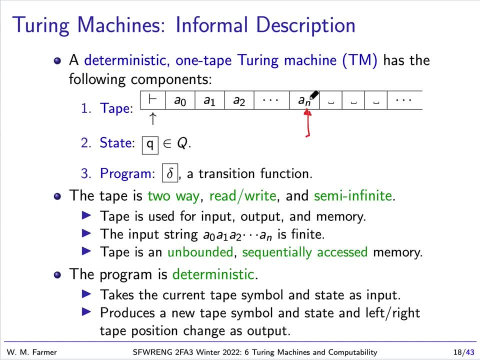 read-write head. it takes the tape symbol, the state, it takes this and the state as input and then it produces a null state. It produces a new tape symbol, let's say B, and a new state, which I'll call P, and then it moves either this way or this way. it moves left or it moves right. 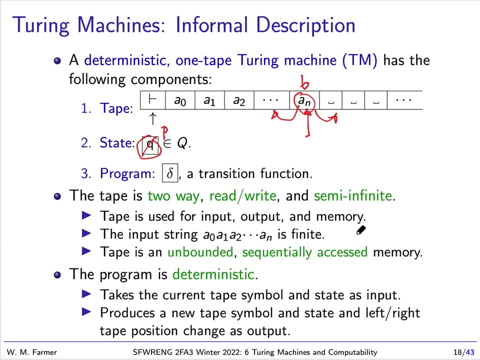 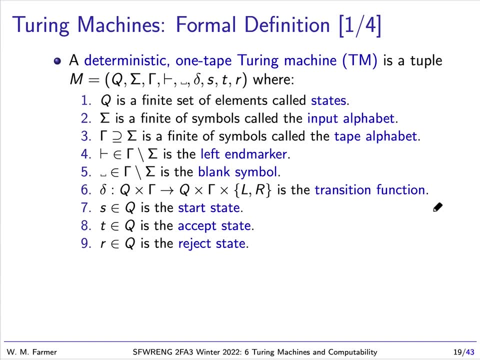 that's basically how the machine works. Okay, so let's look at a formal definition of our deterministic one tape Turing machine, which we'll abbreviate as TM. It's a two-pole, has a nine components. the first component is capital Q. it's a finite set. 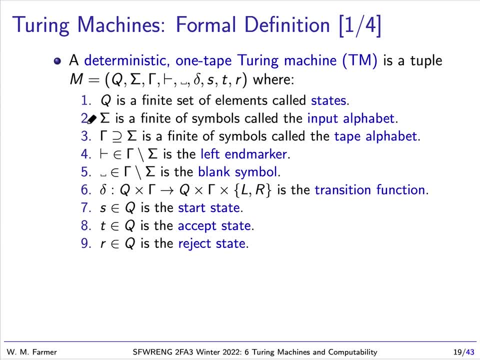 of elements called states. capital sigma is a finite set of symbols called the input alphabet and gamma is a finite. it should be set here: finite set of symbols called the input alphabet and gamma is a finite set of symbols called the input alphabet And the tape alphabet includes it. includes the input alphabet. 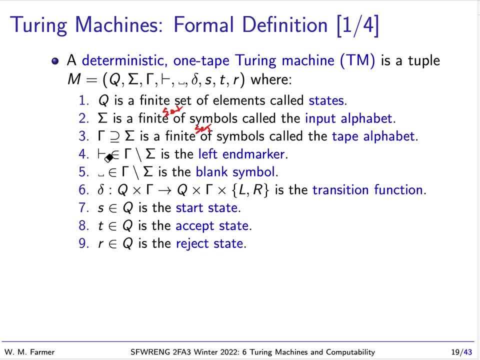 and then there's a special tape symbol, which is not an input symbol, called the left-end marker, which we will denote like this. and then there's a special symbol called the blank symbol, which we will denote like this: And then we have a second symbol, which is the insert symbol. 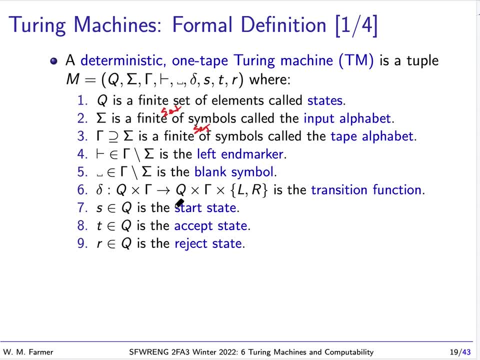 transition function takes a state and a symbol and returns a state and a symbol, and either left or right, and finally we have s is a start state, t is an accept state and r is the reject state. so actually there's one start state, one accept state and one reject state. 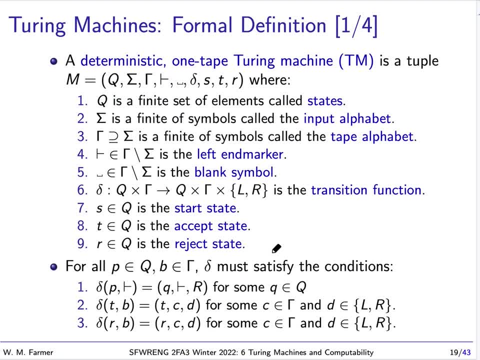 now we have some conditions that delta must satisfy our transition function for all p in q, all b in our tape alphabet. if we're in any state p and we're looking at the leftmost n marker, then we must go to the right. so if we're in any state p and we're looking at the leftmost n marker, then we must go to the right. 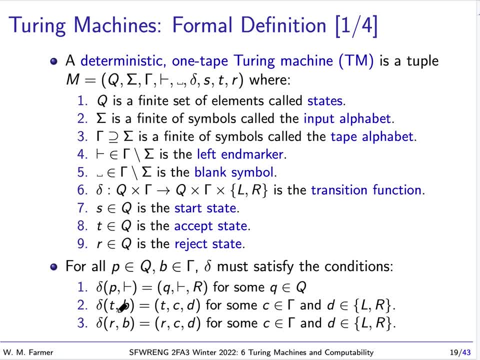 and possibly change the state. and if we're in the accept state t, then whatever we do, we will always remain in the accept state. and if we're in the reject state, whatever we do, we will always remain in the reject state. so, Turing machines, you can think of them as running forever. they always run. 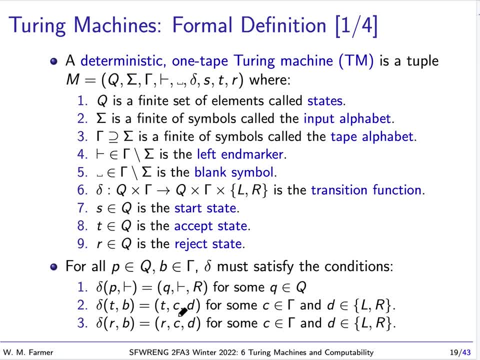 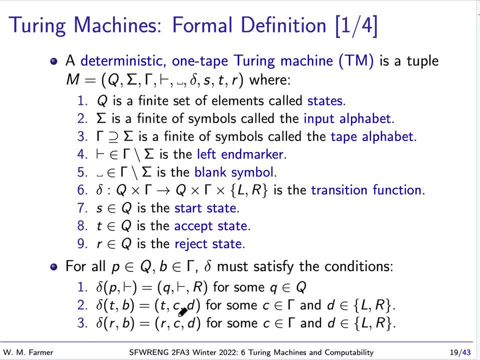 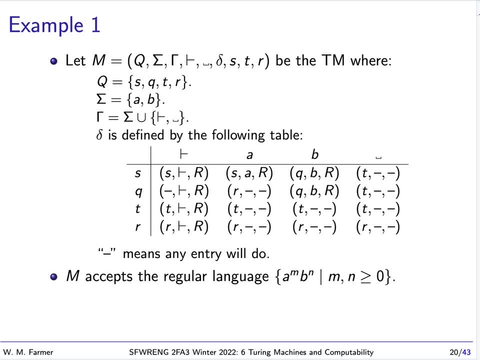 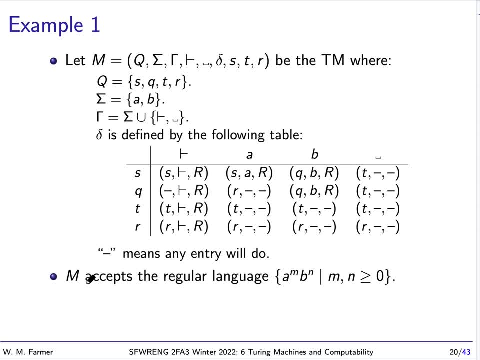 okay, so let's look at a very simple example. okay, so let's look at a very simple example. this is an example. this is an example. this is an example of a Turing machine. m it accepts this of a Turing machine. m it accepts this of a Turing machine. m it accepts this language down here. 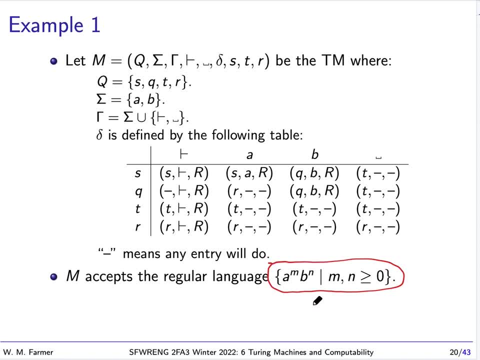 language down here, language down here which you might recognize as a regular, which you might recognize as a regular, which you might recognize as a regular language. this is a very simple language language. this is a very simple language language. this is a very simple language and and we have four states: s, q, t and r. s is a. 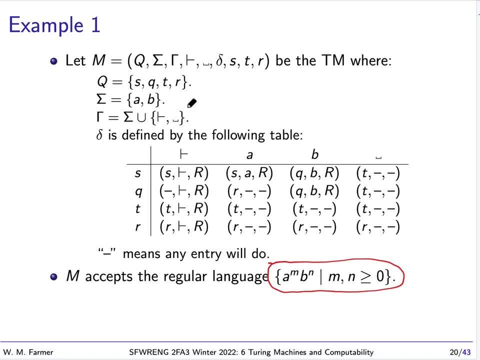 we have four states: s, q, t and r s is a. we have four states: s, q, t and r s is a start state. t is accept. start state: t is accept. start state: t is accept. r is reject and we have two. r is reject and we have two. 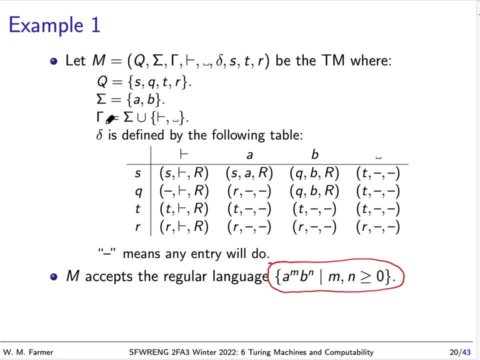 r is reject, and we have two tape symbols and we have one tape symbols and we have one tape symbols and we have one, uh, we have, we have uh for, uh, we have, we have, uh for, uh, we have, we have, uh for, i should say we. a and b are the input. 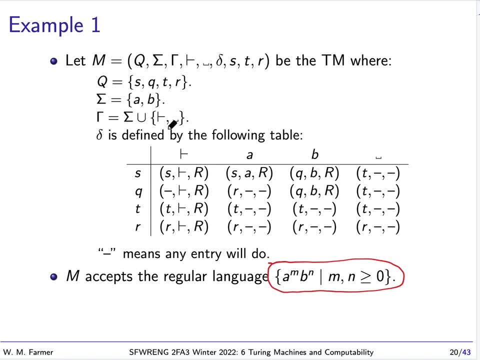 i should say we a and b are the input. i should say we a and b are the input symbols: the tape symbols symbols. the tape symbols symbols. the tape symbols are a and b plus the left end marker, are a and b plus the left end marker, are a and b plus the left end marker and the blank symbol. 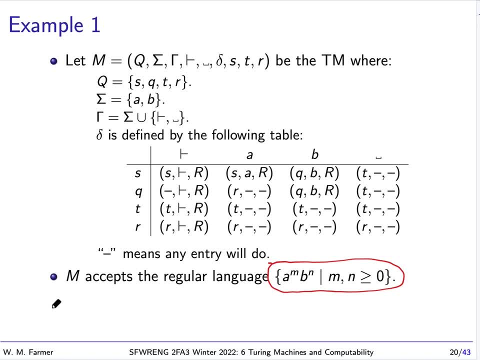 and the blank symbol and the blank symbol, and so let's say we were going to apply this to a string. let's take something very simple. let's say a, a, v. we will start here and we will use this. we'll start here in and we will use this. we'll start here in. 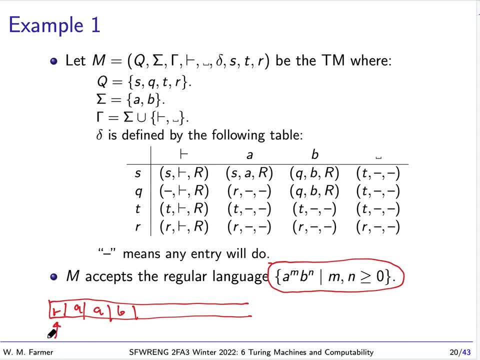 and we will use this. we'll start here in the, the, in the, in, in the, in uh, state s, and so when we're in state s, we're looking at, and so when we're in state s, we're looking at, and so when we're in state s we're looking at this symbol, we'll move to the right. 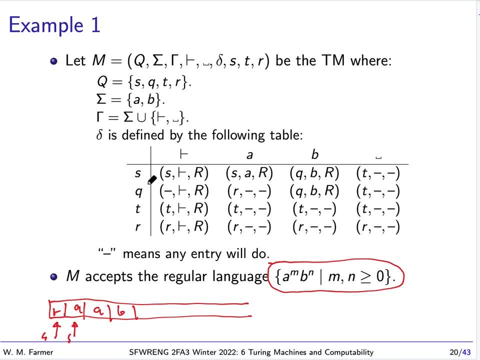 this symbol: we'll move to the right. this symbol: we'll move to the right and stay in s and stay in s and stay in s i should say we're in state s we're. i should say we're in state s we're. i should say we're in state s we're looking at this. 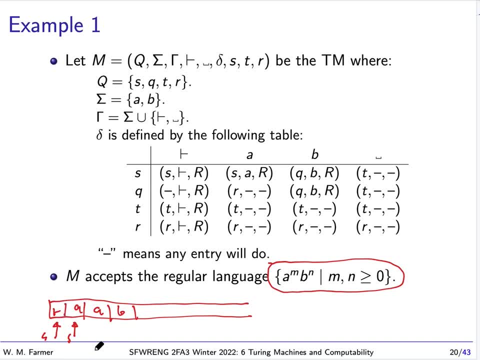 looking at this, looking at this: we will keep this symbol the same, stay in. we will keep this symbol the same, stay in. we will keep this symbol the same, stay in s and move to the right s and move to the right s, and move to the right, and when we move to the right, we'll be. 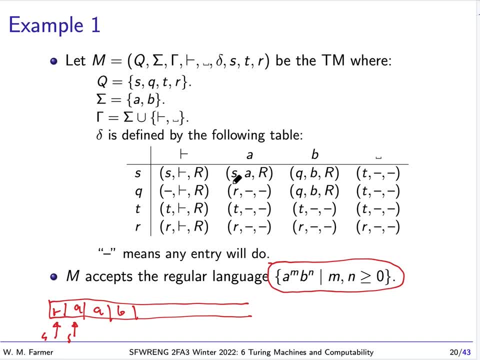 and when we move to the right, we'll be, and when we move to the right, we'll be in state s looking at a, in state s looking at a, in state s looking at a, and we will stay in s and we will stay in s and we will stay in s. we will leave a here and then we move to. 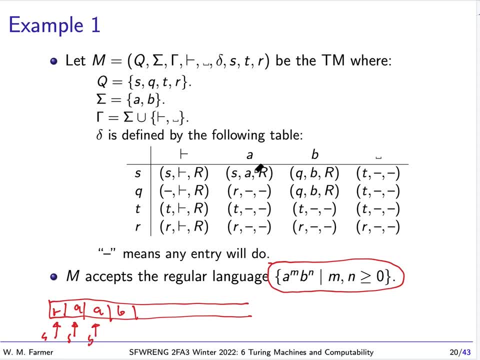 we will leave a here and then we move to. we will leave a here and then we move to the right. and again, same thing will happen, we'll, and again, same thing will happen, we'll, and again, same thing will happen. we'll. move to the right, move to the right. 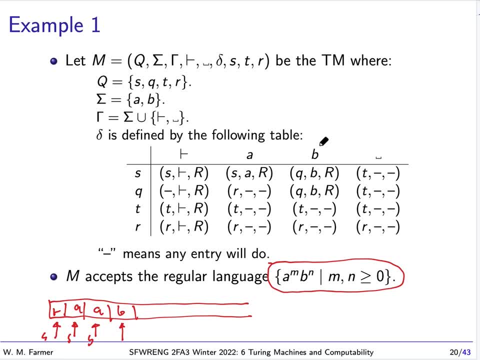 move to the right. and now we're in s, and now we're in s, and now we're in s. we're looking at a- b. we're going to. we're looking at a- b. we're going to. we're looking at a- b. we're going to change a state q. 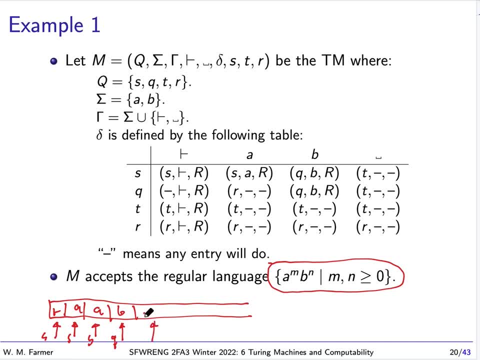 change a state q, change a state q, and we'll move to the right and we'll move to the right and we have blank symbols here and now we're in state q, and now we're in state q, and now we're in state q. we have a blank symbol and we go to the 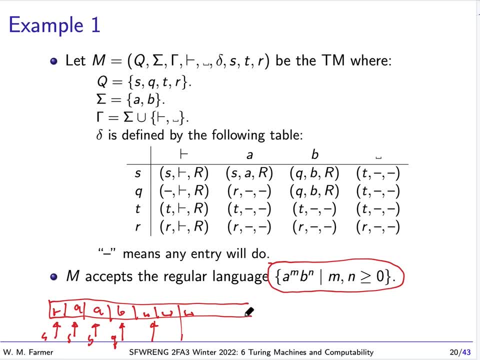 we have a blank symbol and we go to the. we have a blank symbol and we go to the accept state, accept state, accept state. uh, uh, uh, and and and. so therefore, we would accept this, so, therefore, we would accept this, so, therefore, we would accept this, this string. 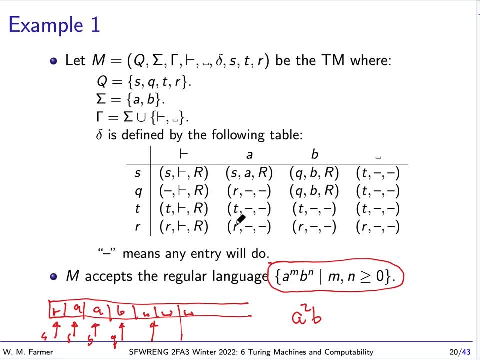 and notice that we're in the accept state. and notice that we're in the accept state and notice that we're in the accept state. it doesn't matter what we do the it doesn't matter what we do the. it doesn't matter what we do the. the dashes here means you can put in any 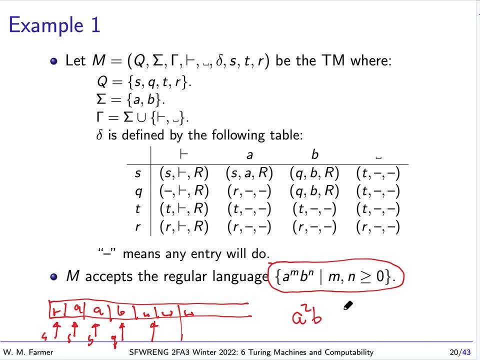 the dashes here means you can put in any. the dashes here means you can put in any information. it doesn't matter. so once information, it doesn't matter. so once information, it doesn't matter. so once we're in the accept state, we always we're in the accept state, we always. 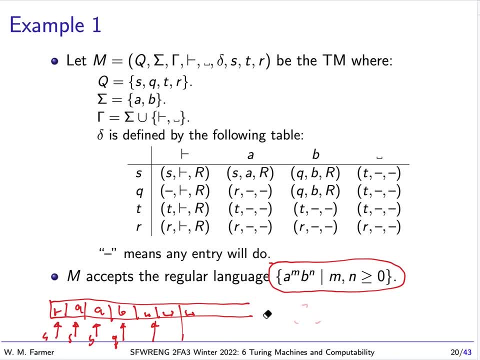 we're in the accept state, we always stay in the accept state. so let's take a stay in the accept state. so let's take a stay in the accept state. so let's take a different example, still a very simple example. let's say we. let's say we. 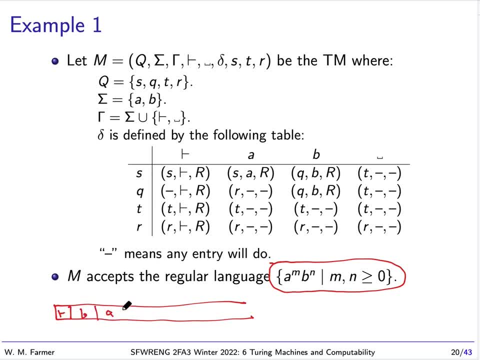 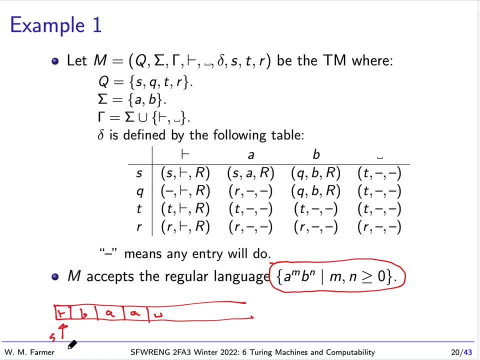 we're in state s we look at this. we're in state s we look at this. we're in state s we're looking at this. we're in state s we're looking at this. we're in state s we're looking at this. we keep this here. we move here, we're. 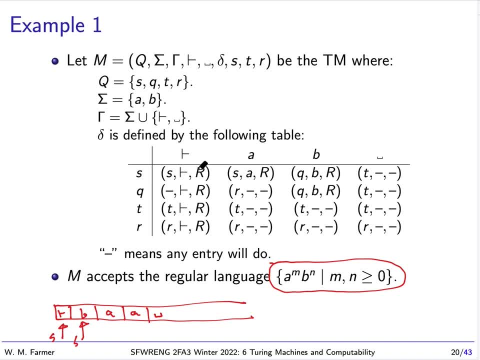 we keep this here, we move here, we're. we keep this here, we move here. we're still in state s, still in state s, still in state s, we're in state s, we're in state s, we're in state s and we move to to the right. 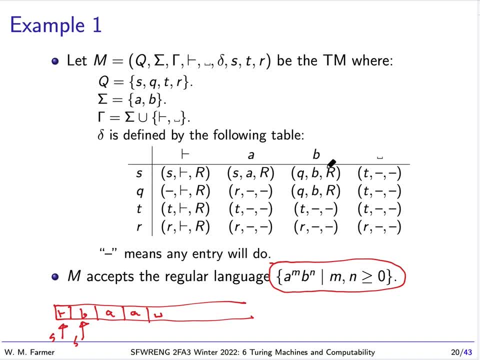 and we move to to the right, and we move to to the right, and now we have a b, and now we have a b, and now we have a b. and what we do when we have a b, we go. and what we do when we have a b, we go. 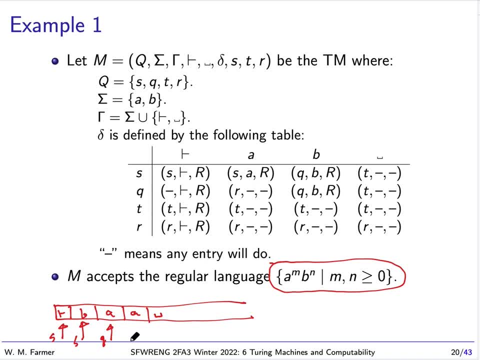 and what we do. when we have a b, we go, we read an a and now we go to the reject. we read an a and now we go to the reject. we read an a and now we go to the reject state, state, state, and then we continue in that reject state. 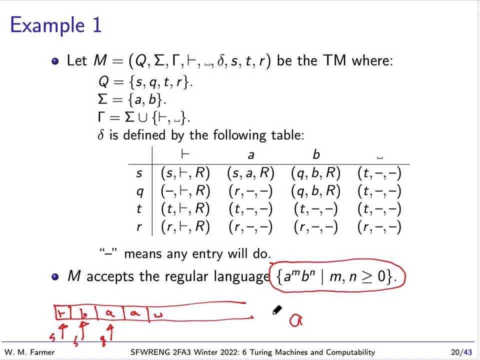 and then we continue in that reject state, and then we continue in that reject state forever, forever, forever. so basically that says that if we have, so basically that says that, if we have, so basically that says that if we have this, this, this, we reject it. it's not a member of that. 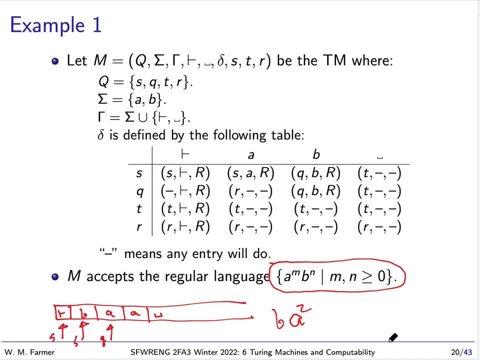 we reject it. it's not a member of that. we reject it. it's not a member of that. okay, so that's a very simple example. okay, so, that's a very simple example. okay, so, that's a very simple example. um, um, um. examples with turing machines can be very 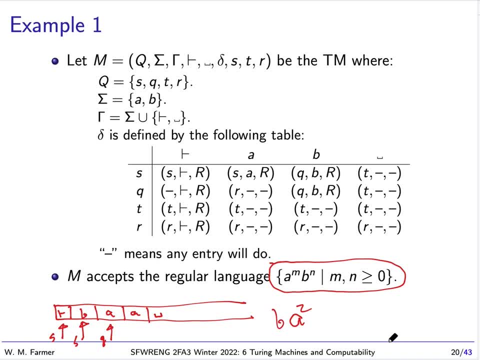 examples with turing machines can be very examples with turing machines can be very complex, complex. complex because these machines are are quite, because these machines are are quite, because these machines are are quite powerful, powerful, powerful. we can go back and forth on the tape we. we can go back and forth on the tape we. 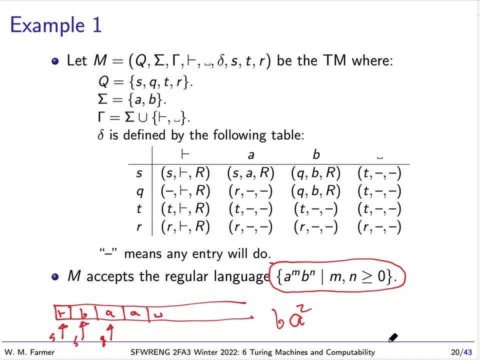 we can go back and forth on the tape. we can write down whatever we want on the can write down whatever we want on the can write down whatever we want on the tape, tape, tape. the tape is infinite to the right, so we. the tape is infinite to the right, so we. 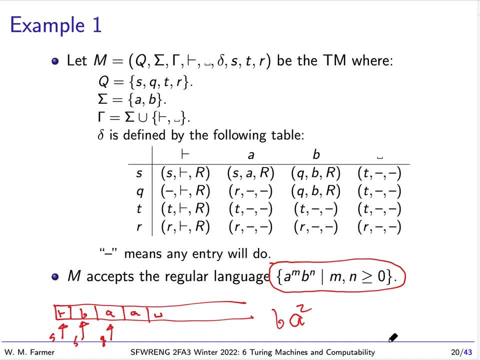 the tape is infinite to the right, so we have lots of space to work, have lots of space to work, have lots of space to work. so there's great power here. so there's great power here. so there's great power here and, as a result, if we're going to do, 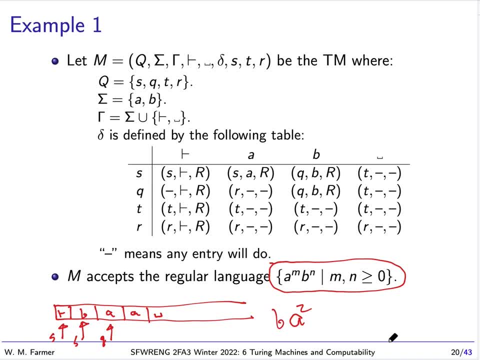 and, as a result, if we're going to do, and, as a result, if we're going to do, something sophisticated with a turing, something sophisticated with a turing, something sophisticated with a turing machine, machine, machine, the transition function is likely to be. the transition function is likely to be. 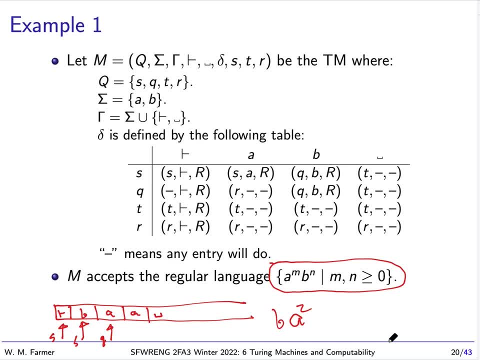 the transition function is likely to be very big and complicated. okay, so i have a question for you. a okay, so i have a question for you. a okay, so i have a question for you. a turing machine will either accept or turing machine will either accept or. 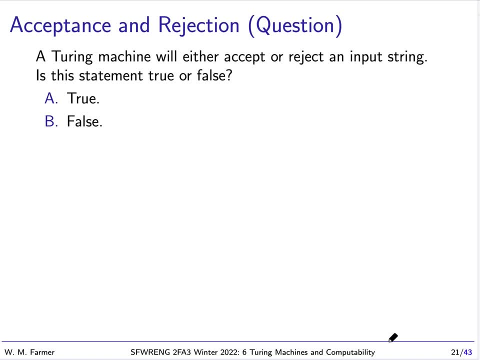 turing machine will either accept or reject an input string. is this statement reject an input string? is this statement reject an input string? is this statement true or false? true or false, true or false. so i'll give you a moment to think about. so i'll give you a moment to think about. 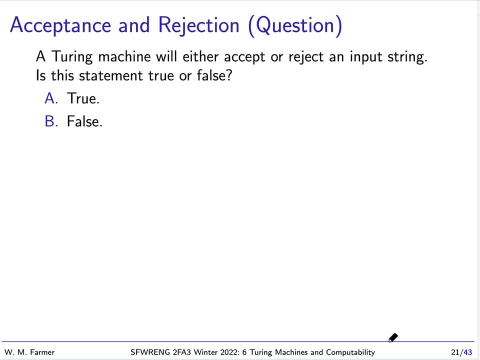 so i'll give you a moment to think about this. well, welcome back. actually it is false. well, welcome back, actually it is false. well, welcome back. actually it is false. because a turing machine has three, because a turing machine has three, because a turing machine has three possibilities. 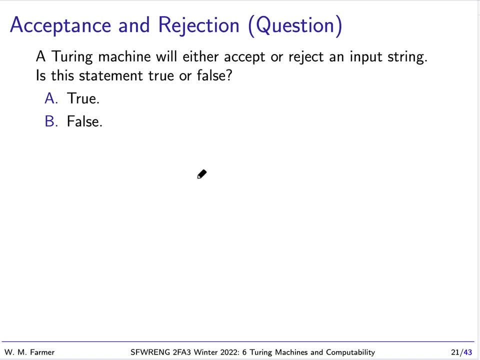 possibilities, possibilities. when you run it on a string, it can go. when you run it on a string, it can go. when you run it on a string, it can go to the accept, into the accept state, to the accept, into the accept state, to the accept, into the accept state. therefore, it accepts or it can go into. 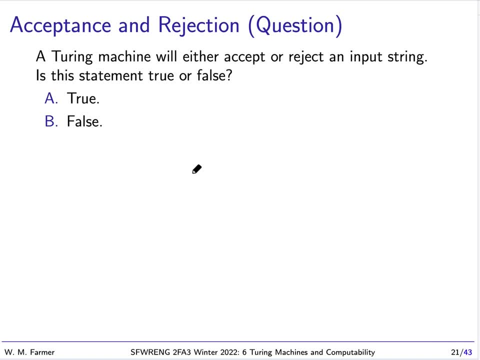 therefore it accepts or it can go into. therefore it accepts or it can go into the reject state. therefore it rejects the reject state. therefore it rejects the reject state. therefore it rejects: or it may never reach either the accept, or it may never reach either the accept, or it may never reach either the accept state or the reject state. 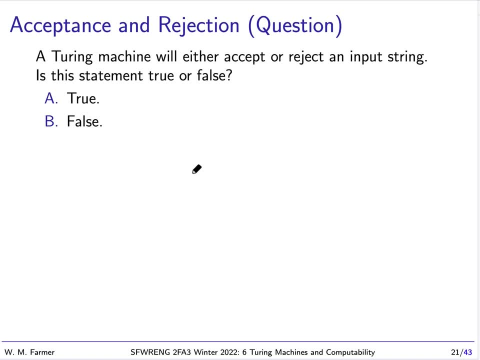 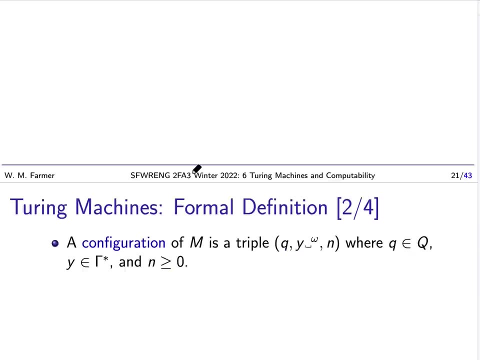 state or the reject state. state or the reject state, the turing machine just runs forever. the turing machine just runs forever. the turing machine just runs forever. so turing machines have these three. so turing machines have these three. so turing machines have these three possibilities. 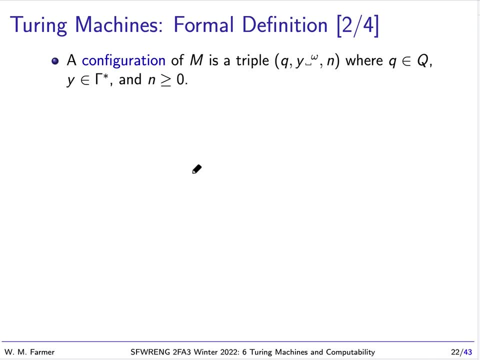 okay, so let's continue talking about. okay, so, let's continue talking about. okay, so, let's continue talking about turing machines, turing machines, turing machines. a configuration, a configuration. a configuration looks like this. it has a state. looks like this. it has a state, looks like this. it has a state here. 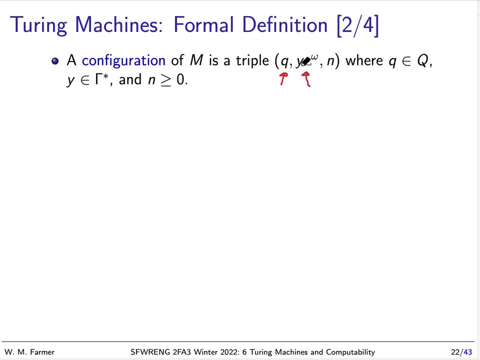 it has what's on, it has what's on, it has what's on the tape, and that will always be a the tape, and that will always be a the tape, and that will always be a string of input symbols. string of input symbols. string of input symbols followed by. 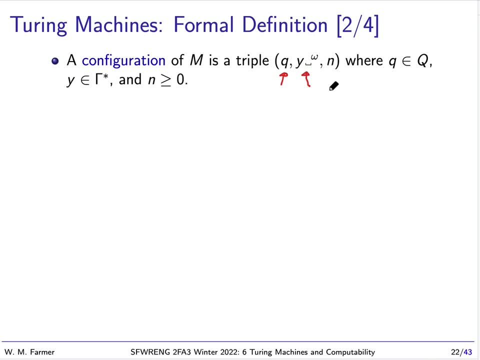 followed by, followed by an, an, an infinite sequence of blank, infinite sequence of blank. infinite sequence of blank sequence. infinite sequence of blank sequence. symbols, symbols, symbols, and then there will be a natural number, and then there will be a natural number, and then there will be a natural number n. 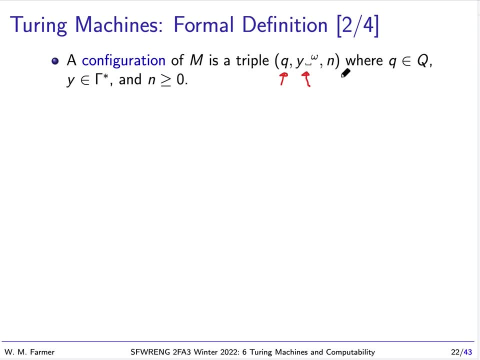 n, n, and that will be the position where the and that will be the position where the and that will be the position where the read write head is at now. this configuration describes now. this configuration describes now. this configuration describes the machine in state q. the machine in state q. 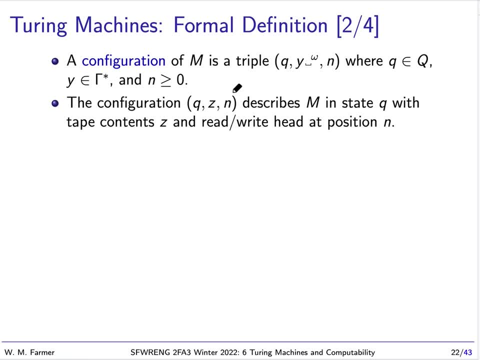 the machine in state q. it has contents z and the rewrite head it has contents z and the rewrite head it has contents z and the rewrite head is that position in. and we're going to denote configurations by: and we're going to denote configurations by: and we're going to denote configurations by greek. 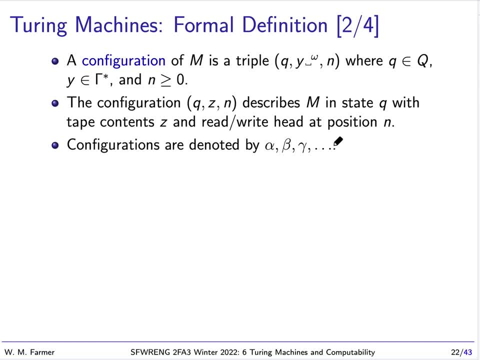 greek: greek: greek letters starting in the beginning of the letters, starting in the beginning of the letters, starting in the beginning of the greek alphabet, greek alphabet, greek alphabet. so in this case, alpha beta gamma. so in this case, alpha beta gamma. so in this case, alpha beta gamma and the start configuration as we've. 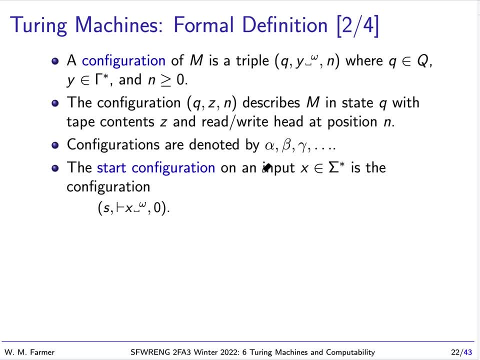 and the start configuration, as we've and the start configuration, as we've already seen, already seen, already seen, is is going to be the start, is is going to be the start, is is going to be the start. configuration on a particular input: x is. configuration on a particular input: x is. 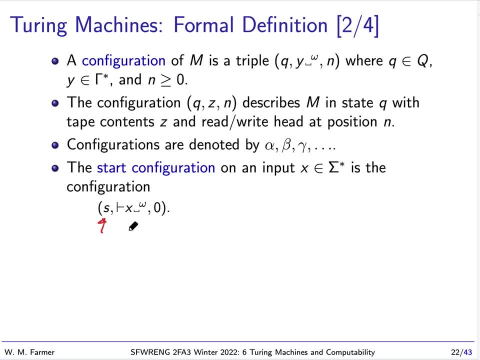 configuration on a particular input. x is going to look like this, going to look like this, going to look like this. this is the start state. the contents of this is the start state. the contents of this is the start state. the contents of the tape will be. the tape will be. 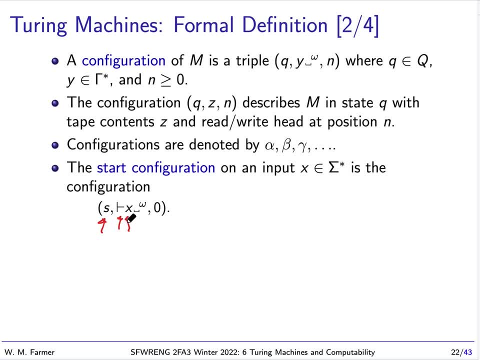 the tape will be the left end marker, the string, the input, and then this infinite sequence of input, and then this infinite sequence of input, and then this infinite sequence of blank symbols, blank symbols, blank symbols. and we're going to be reading, and we're going to be reading. 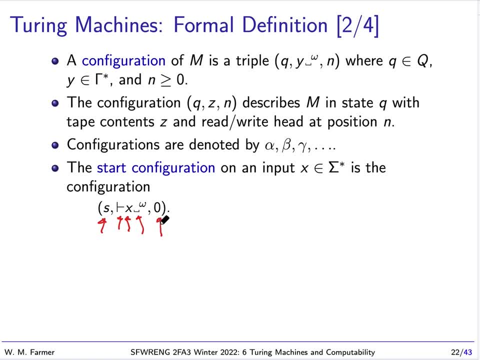 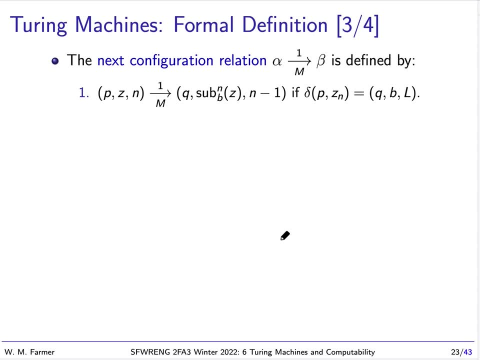 and we're going to be reading the zeroth. or this will be the first, the zeroth, or this will be the first the zeroth, or this will be the first entry and the tape. now we can define the. now we can define the. now we can define the next configuration relation. 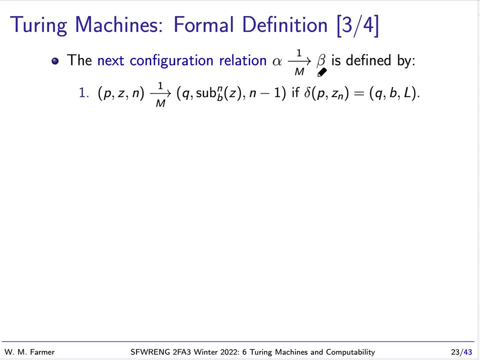 next configuration relation. next configuration relation. so how do we get from configuration? so how do we get from configuration? so how do we get from configuration? alpha to beta. how do we do go to the alpha to beta? how do we do go to the alpha to beta? how do we do go to the next? one is defined as follows: if we 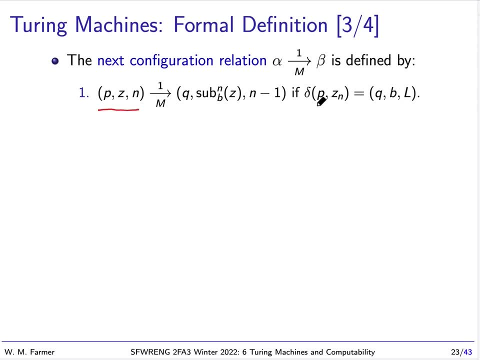 next one is defined as follows: if we next one is defined as follows: if we have this configuration, have this configuration, have this configuration, and we have our this and we have our this and we have our this in our um, our transition function, in our um, our transition function. 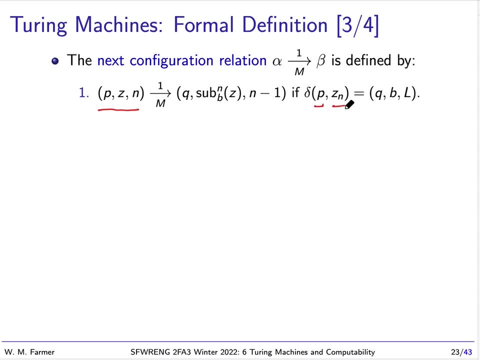 in our um, our transition function. so we have p here looking at. so we have p here looking at. so we have p here looking at zn. zn is the nth member of this string z here see. string z here see. string z here see in the in the. 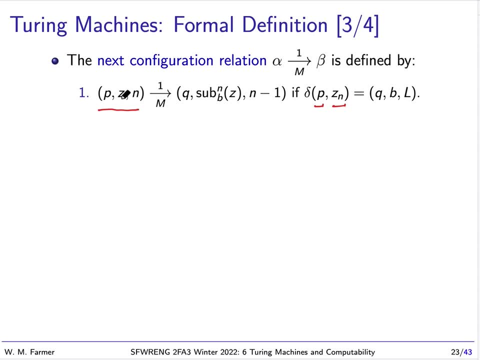 in the, in this configuration, the readhead, in this configuration, the readhead, in this configuration, the readhead: rewrite head is then rewrite head, is then rewrite head, is then the nth position. and if we have this, the nth position, and if we have this, the nth position, and if we have this transition, we're going to go to q. 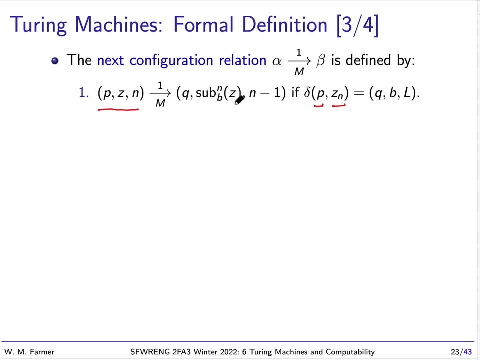 transition. we're going to go to q transition, we're going to go to q bl. so this will change the q bl, so this will change the q bl, so this will change the q and we will replace, and we will replace, and we will replace in z the nth. 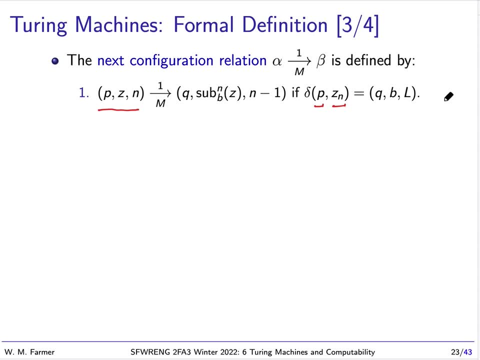 in z the nth. in z the nth, we'll replace the nth position with b. we'll replace the nth position with b. we'll replace the nth position with b, and then we'll move to the left, which, and then we'll move to the left which, and then we'll move to the left, which means we'll change the position of the. 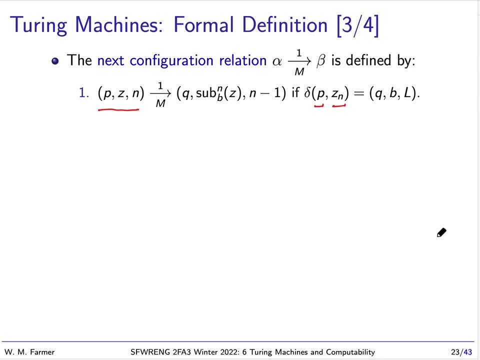 means we'll change the position of the means, we'll change the position of the read write head, read, write head, read, write head to n minus one. so that's how that works- to n minus one. so that's how that works to n minus one. so that's how that works, and we have something quite similar. 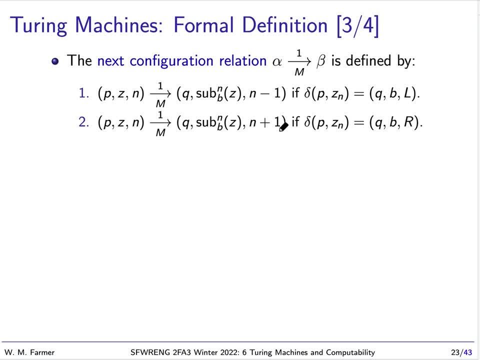 and we have something quite similar. and we have something quite similar. if this is r, in that case the read. if this is r, in that case the read. if this is r, in that case the read: write head, write head, write head is incremented by one, and then we can define. 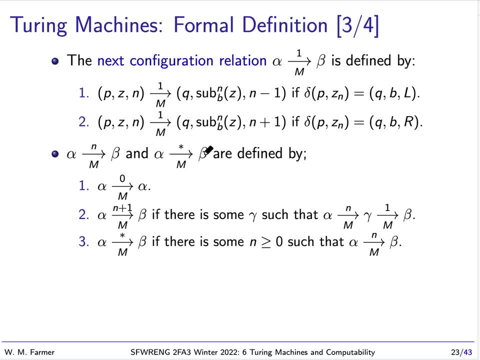 this relation for n steps or for any. this relation for n steps or for any. this relation for n steps or for any number of steps. number of steps. number of steps. so zero steps, so zero steps, so zero steps. we go from the configuration to itself. we go from the configuration to itself. 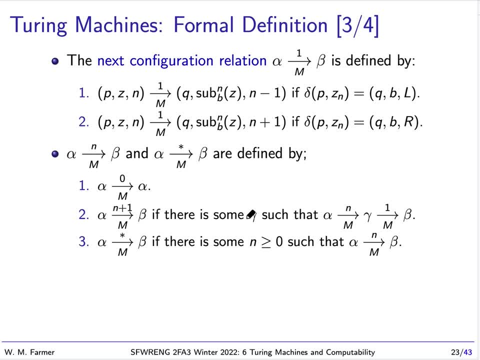 we go from the configuration to itself. if we're going n plus one steps. if we're going n plus one steps. if we're going n plus one steps, what that means is there's some way we. what that means is there's some way we. what that means is there's some way we can. 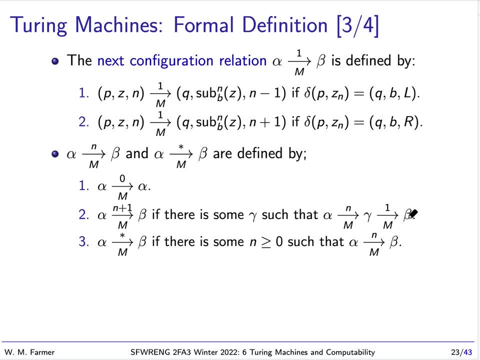 can, can go n steps, then followed by go n steps, then followed by go n steps, then followed by one step, and one step and one step. and if we have star, that just means there's. if we have star, that just means there's. if we have star, that just means there's some number of steps. 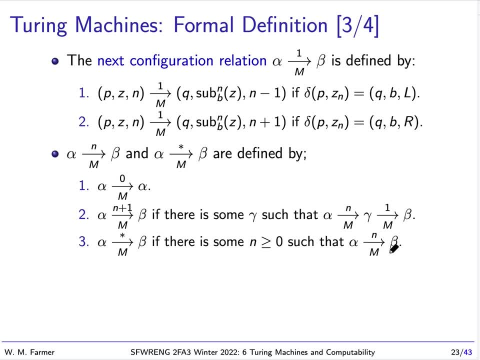 some number of steps, some number of steps n greater than equal to zero. so we go n greater than equal to zero, so we go n greater than equal to zero, so we go from alpha to beta, from alpha to beta, from alpha to beta, and, as we've talked about before this: 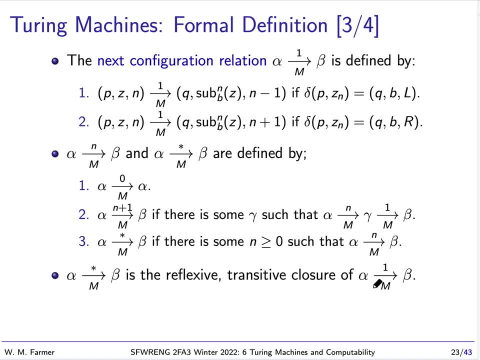 and, as we've talked about before this and as we've talked about before this relation, star relation is reflexive relation. star relation is reflexive relation. star relation is reflexive transitive closure of our next transitive closure of our next transitive closure of our next configuration relation. 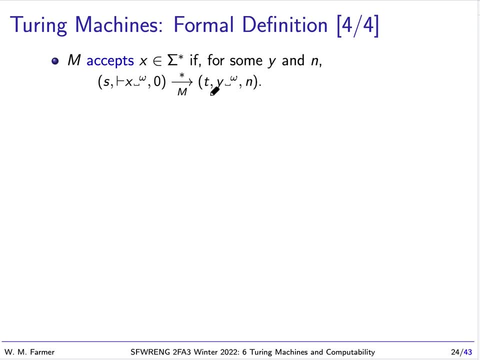 now m accepts the string. now m accepts the string. now m accepts the string: if, if we, if there's a transition, if, if we, if there's a transition, if, if we, if there's a transition from the initial configuration, from the initial configuration, from the initial configuration to some configuration. 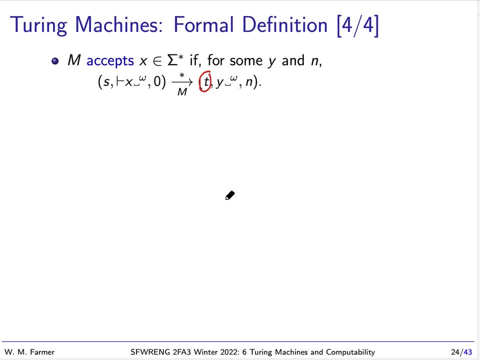 to some configuration, to some configuration where the state, where the state, where the state is the accept state, so it can be any is the accept state, so it can be. any is the accept state, so it can be any configuration, configuration, configuration, as long as we can get to the accept state. 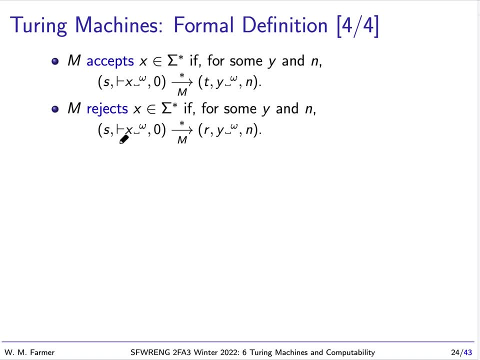 as long as we can get to the accept state. as long as we can get to the accept state. and and. and. m rejects a string similarly we. m rejects a string. similarly we. m rejects a string similarly: we. there's some transition from. there's some transition from. 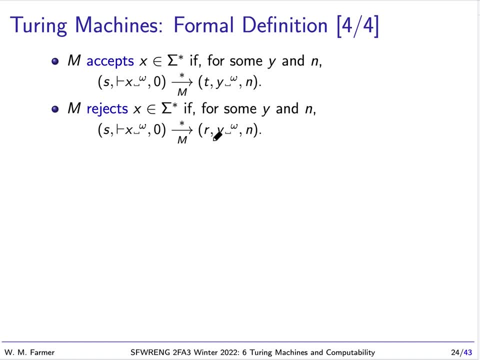 there's some transition from the start configuration, the start configuration, the start configuration, to a configuration where we have to a configuration where we have to a configuration where we have the reject state, and so we'll say m halts on x, and so we'll say m halts on x. 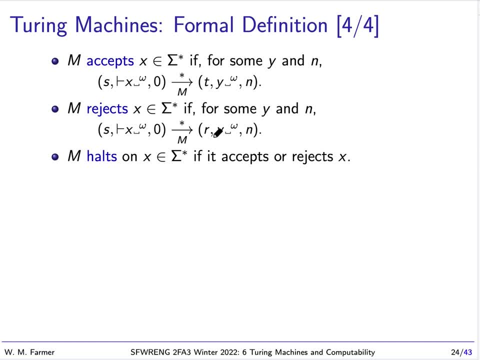 and so we'll say: m halts on x if it either accepts. if it either accepts, if it either accepts or rejects x, that means it either. or rejects x, that means it either. or rejects x, that means it either enters the accept state or reject state, and we'll say m loops on x if it neither. 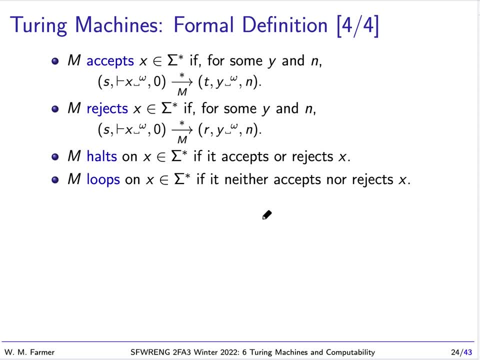 and we'll say m loops on x if it neither. and we'll say m loops on x if it neither accepts nor rejects x accepts nor rejects x accepts nor rejects x. it just runs forever. never getting to. it just runs forever. never getting to. it just runs forever. never getting to the accept or reject state. 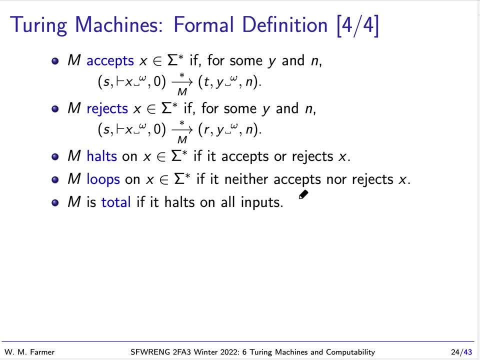 the accept or reject state. the accept or reject state and we'll say m is total if it halts in. and we'll say m is total if it halts in. and we'll say m is total if it halts in all inputs and we'll let l of m be the set of. 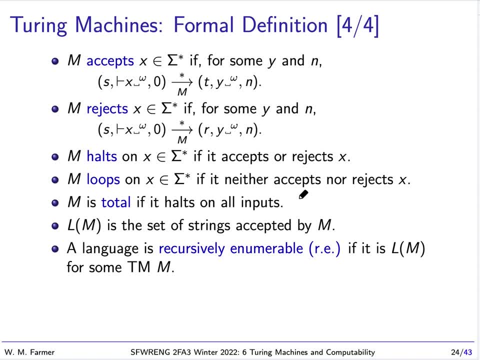 and we'll let l of m be the set of and we'll let l of m be the set of strings accepted by m, strings accepted by m, strings accepted by m, and we will say a language is, and we will say a language is, and we will say a language is recursively enumerable. re for short. 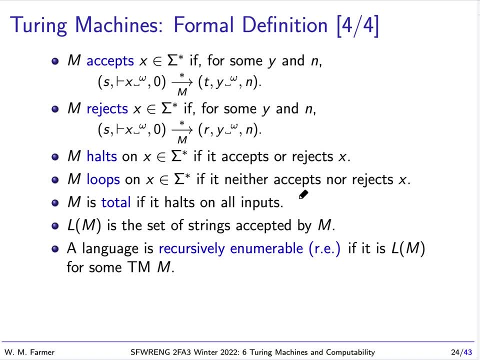 recursively enumerable re for short. recursively enumerable re for short, if it is, if it is the language for some, if it is, if it is the language for some, if it is, if it is the language for some: turing machine, so turing machines. turing machine, so turing machines. 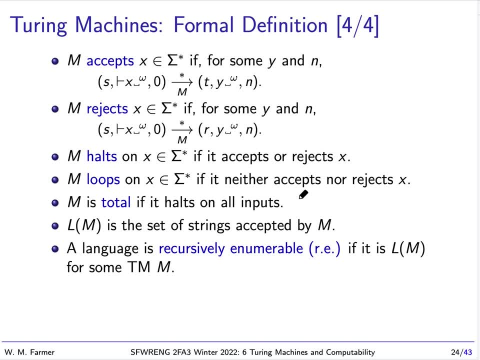 turing machine. so turing machines in general. they accept recursively in general. they accept recursively in general. they accept recursively enumerable languages, enumerable languages, enumerable languages and a language is recursive and a language is recursive and a language is recursive if it is the language for some total. 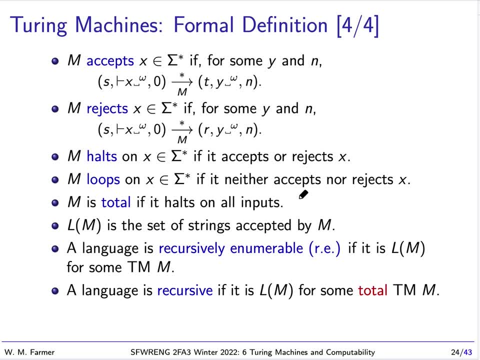 if it is the language for some total, if it is the language for some total turing machine, so total turing machines, turing machine, so total turing machines, turing machine, so total turing machines. accept. accept. accept. recursive languages, so the recursive languages, so the. 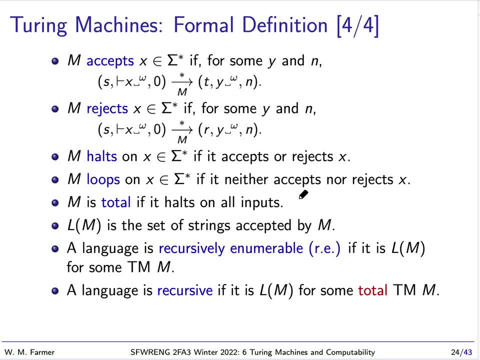 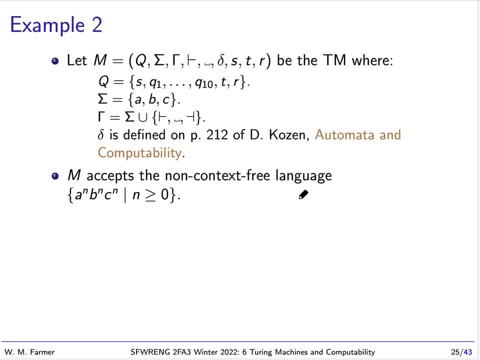 recursive languages. so the recursively enumerable languages include recursively enumerable languages, include recursively enumerable languages, include the recursive languages, the recursive languages, but not every recursive language is the recursive languages, but not every recursive language is the recursive languages, but not every recursive language is recursively enumerable, recursively enumerable, recursively enumerable. okay, so let's look at a second example. 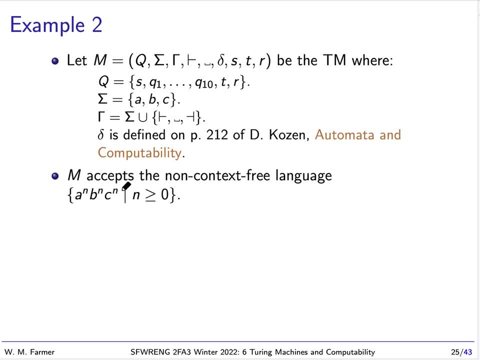 okay, so let's look at a second example. okay, so let's look at a second example. this is much more interesting than our. this is much more interesting than our. this is much more interesting than our first example. first example, first example: this is a machine that accepts a non-context. 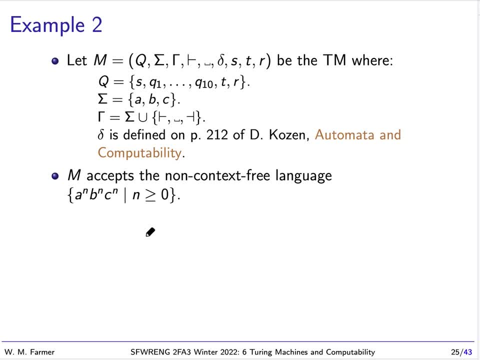 this is a machine that accepts a non-context. this is a machine that accepts a non-context free language. free language. free language. a to the n. b, the n, c, the n where n is a to the n. b, the n. c. the n where n is a to the n. b, the n. c, the n where n is greater than or equal to zero. 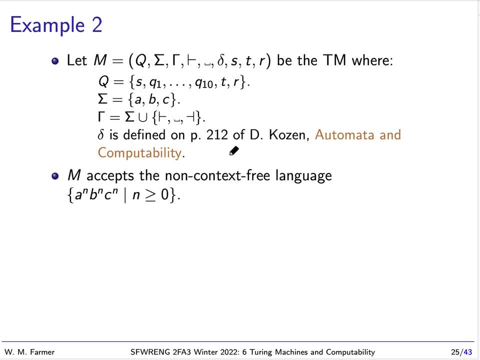 greater than or equal to zero, greater than or equal to zero. i'm not actually going to give you the, i'm not actually going to give you the, i'm not actually going to give you the details, details, details of this machine, but of this machine, but of this machine, but it has these. 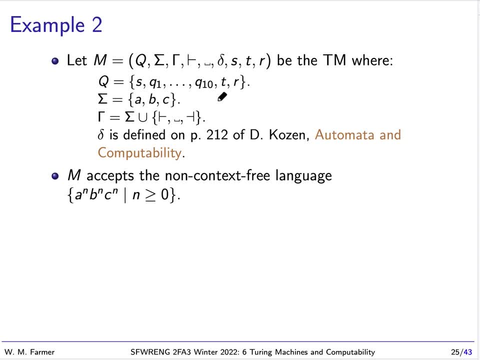 it has these, it has these states, has a start state, then in states, has a start state, then in states, has a start state, then in addition, has addition, has states, has a start state, then in addition, has ten other states and it has ten other states and it has. 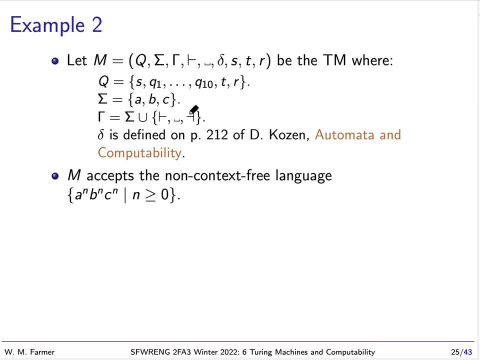 ten other states and it has an accept and reject state. its an accept and reject state. its an accept and reject state. its input: alphabet: input: alphabet input alphabet is a, b and c is a, b and c is a, b and c, and it has and it has. 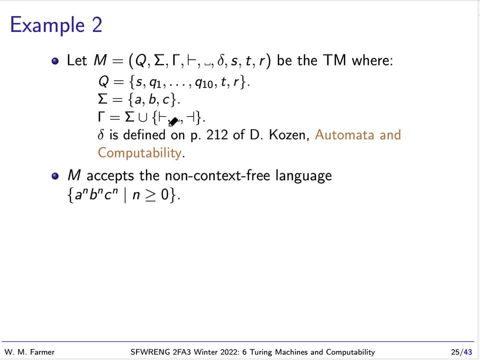 and it has, in addition to the input alphabet, for, in addition to the input alphabet, for, in addition to the input alphabet for its state alphabet, it has its state alphabet. it has its state alphabet. it has the left end marker. it also has a right, the left end marker. it also has a right. 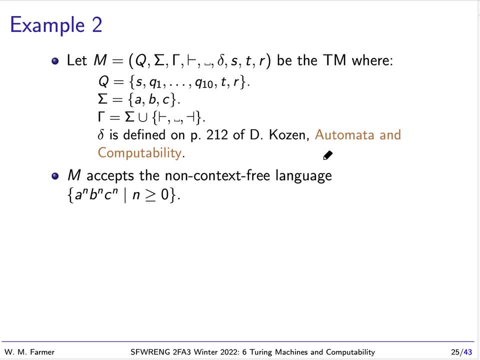 the left end marker. it also has a right end marker and it has a blank symbol end marker and it has a blank symbol end marker and it has a blank symbol and you can find the details for this and you can find the details for this and you can find the details for this machine on page 212 of dexter cosin's. 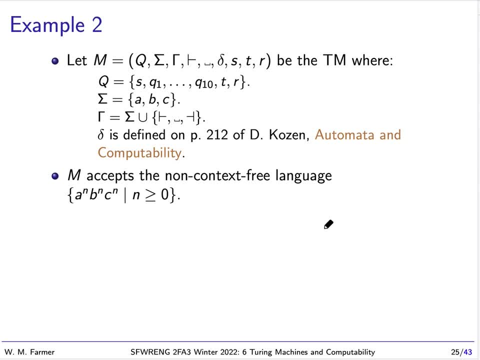 machine on page 212 of dexter cosin's machine. on page 212 of dexter cosin's book automata and computability. book automata and computability. book automata and computability. now we can describe how this works. now we can describe how this works. 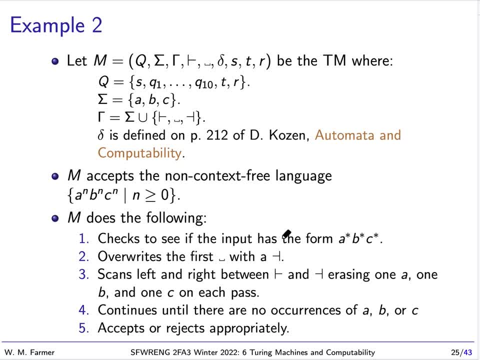 now we can describe how this works and i think you can be convinced, we and i think you can be convinced, we and i think you can be convinced we could actually write down, could actually write down, could actually write down a transition function. that would a transition function, that would. 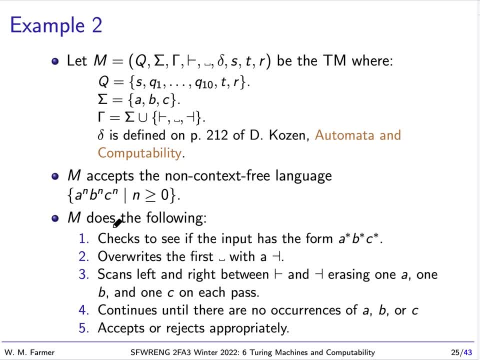 a transition function that would make this machine work as described. make this machine work as described. make this machine work as described. so what m does, so what m does. so what m does, it's going to start at the leftmost. it's going to start at the leftmost. 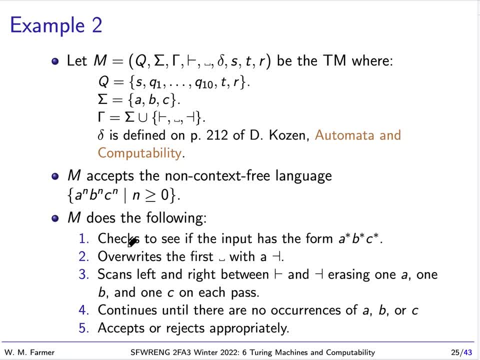 it's going to start at the leftmost symbol, the left end marker symbol, the left end marker symbol, the left end marker, and it's going to move to the right and it's going to move to the right and it's going to move to the right and it's going to check that the input. 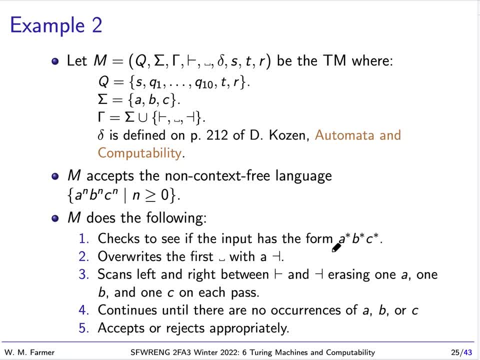 and it's going to check that the input and it's going to check that the input has the form, has the form, has the form: a star, b star, c star. so it's going to a star, b star, c star. so it's going to a star b star, c star. so it's going to make sure the first thing that it's make sure the first thing that it's make sure the first thing that it's going to be reading is an a and it going to be reading is an a and it going to be reading is an a and it reads a bunch of a's and it goes to. 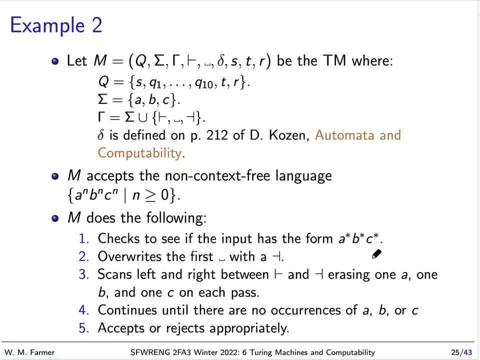 reads a bunch of a's and it goes to reads a bunch of a's and it goes to reading a bunch of b's and reading a bunch of b's and reading a bunch of b's and reading a bunch of c's and finally reading a bunch of c's and finally. 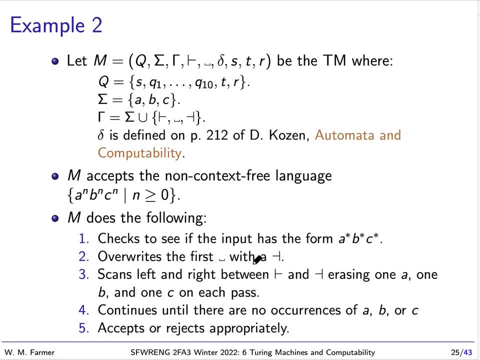 reading a bunch of c's and finally it's going to end up with a blank symbol. it's going to end up with a blank symbol. it's going to end up with a blank symbol. it will overwrite that blank symbol. it will overwrite that blank symbol. it will overwrite that blank symbol with a right end marker. 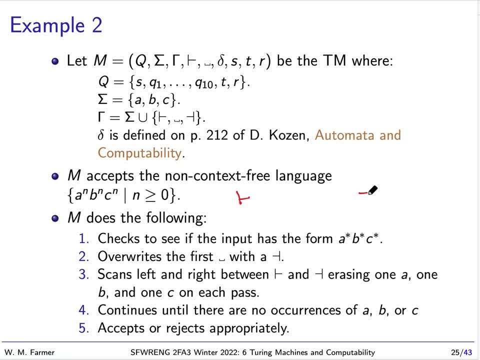 with a right end marker, with a right end marker. so that means it's going to have. so that means it's going to have. so that means it's going to have something here and in here it's going to something here and in here it's going to. 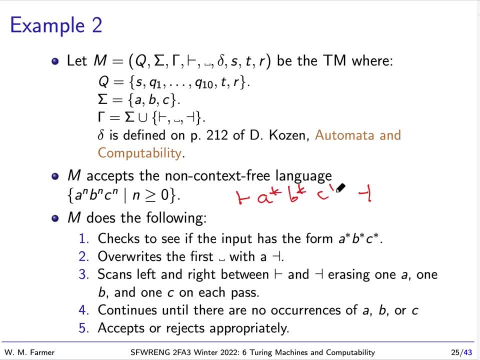 something here and in here it's going to be a bunch of a's, be a bunch of a's, a bunch of b's and a bunch of c's, a bunch of b's and a bunch of c's, a bunch of b's and a bunch of c's. and then what it does, it scans back and 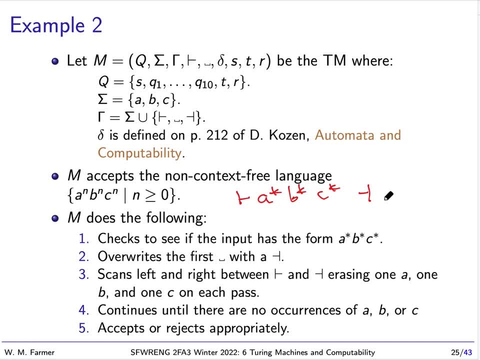 and then what it does? it scans back, and. and then what it does? it scans back and forth, forth, forth. so it scans left and right between these, so it scans left and right between these, so it scans left and right between these two, two, two, and when, um each to each pass it. 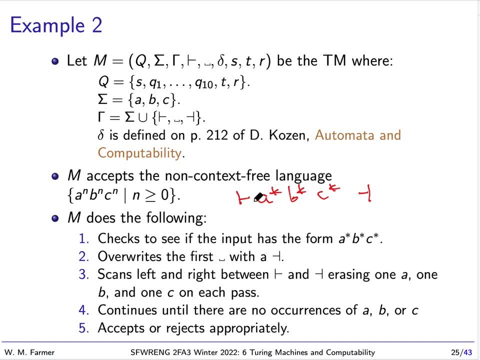 and when um each to each pass it and when um each to each pass. it depends how we want to do it. we could depends how we want to do it. we could depends how we want to do it. we could just always go back here and start. just always go back here and start. 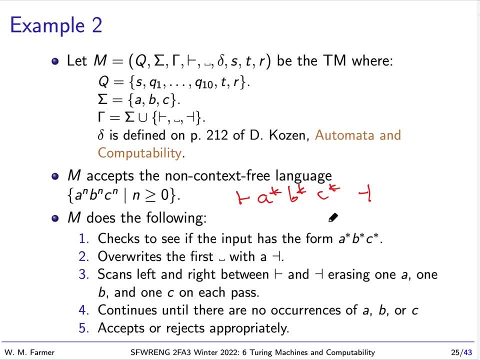 just always go back here and start: it's going to erase a a. it will erase a. it's going to erase a a, it will erase a. it's going to erase a a. it will erase a, b, and then it will erase a c, b and then it will erase a c. 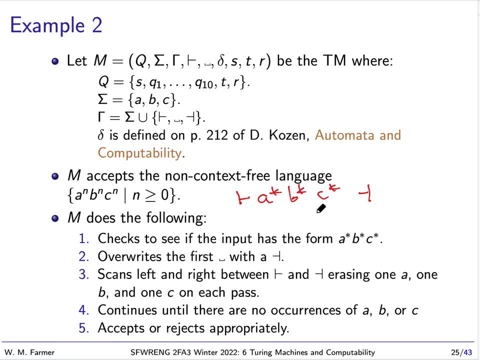 b, and then it will erase a c, go back here again. erase an a, erase a b. go back here again. erase an a, erase a b. go back here again. erase an a, erase a b, erase a c. it will continue doing that. erase a c. it will continue doing that. 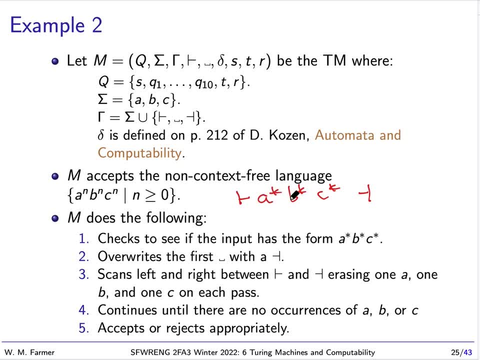 erase a, c, it will continue doing that until there are no occurrences. until there are no occurrences, until there are no occurrences of a, b and c to erase anymore of a, b and c to erase anymore of a, b and c to erase anymore, and in that case it will accept. but if 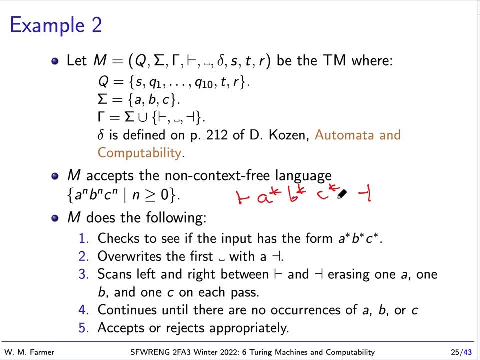 and in that case it will accept. but if, and in that case it will accept. but if it turns out, it turns out, it turns out it. there isn't a symbol that neat that it. there isn't a symbol that neat that it. there isn't a symbol that neat that can be erased. let's say: 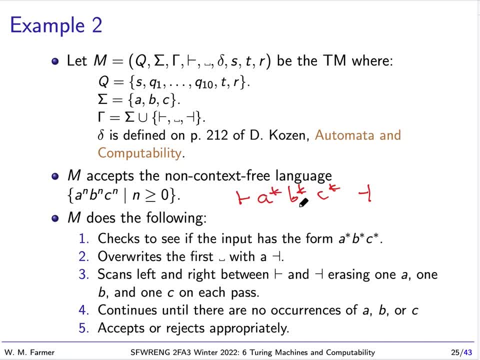 can be erased. let's say: can be erased. let's say it erased an a and now there's no b to it. erased an a and now there's no b to it. erased an a and now there's no b to erase, erase, erase. then it would reject. so that's how this.